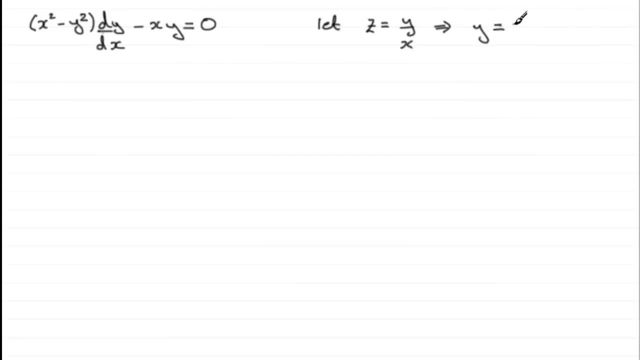 So we get: Y equals X times Z. OK, So if we need to change dy by dx, we need to differentiate this equation with respect to X, And that means that, therefore, dy by dx is going to equal. well, we need to use the product rule for this particular part here. 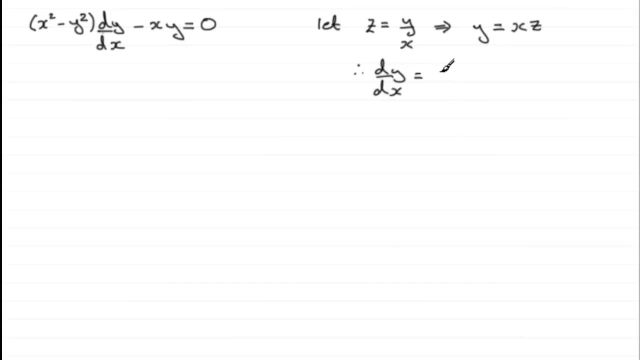 So we take X, for instance, and multiply it by the differential of Z with respect to Z With respect to X. that's going to be dz, dx, And then plus, and then we take the Z and we multiply it by the differential of X with respect to X, which is 1.. 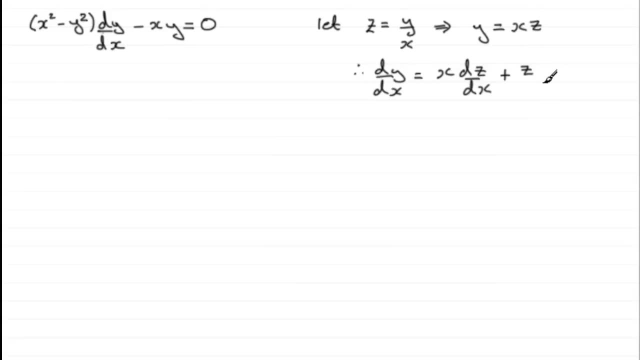 Z times 1 then is just simply Z. So that's dy by dx, And you're going to quite often find that you're going to need to do something along these kind of lines. Use the product rule. So I hope you've got the kind of idea. 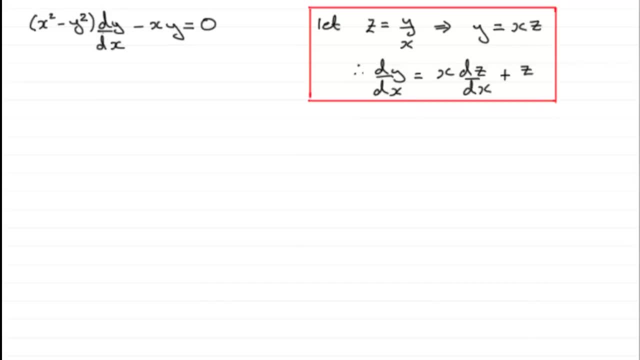 Of how to go about that. OK, So we're now ready to do some substitutions. So for the first bracket here we therefore have X squared. OK, Let's just put that in brackets here, Minus Y squared, But Y equals X times Z. 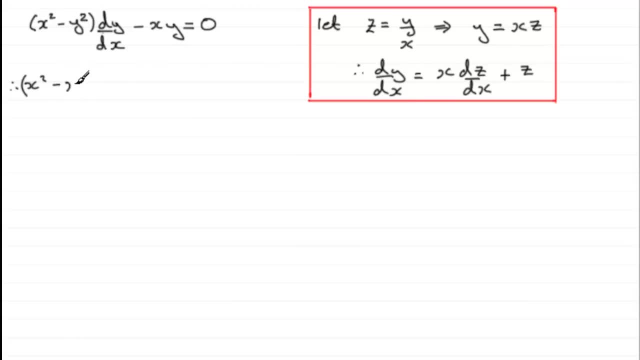 So if we square that, that's going to be minus X squared, Z squared. And then we've got to multiply it by dy, by dx. So we've got to multiply it by dy by dx, So that is now going to be X dz by dx plus Z. 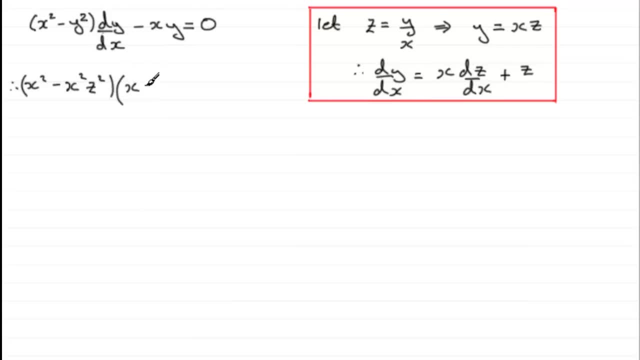 So we'll just put that in brackets: So X dz by dx plus Z, And then we've got minus X Y, So minus X, But Y is X Z. So we've just got multiply by X Z And that equals zero. 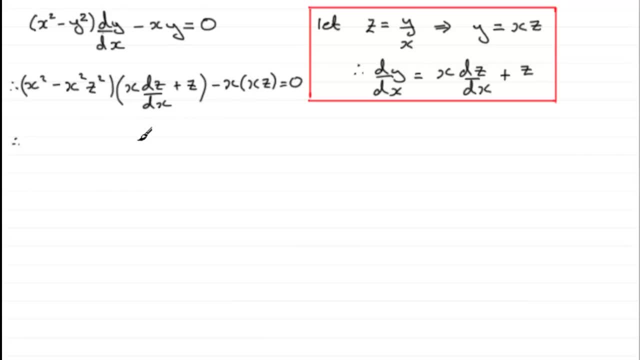 OK. Next, What I'd want to do is start to expand the bracket here. So we've got X squared, then times X, dz dx. That's going to give us X cubed dz by dx. And then we've got X squared, times the plus Z. 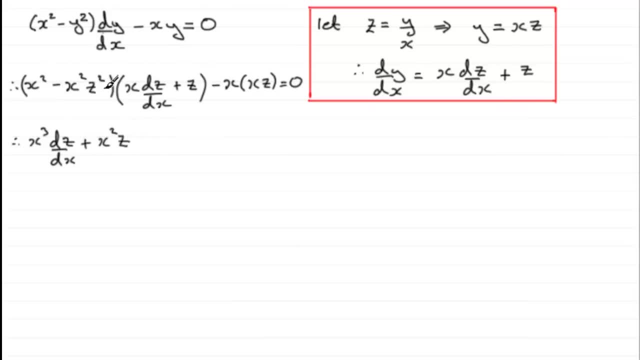 So X squared Z. Now we've got minus X, squared Z, squared times: X, dz, dx, That's going to be minus X, cubed Z squared. And then we've got this last term here: minus X, squared Z. And finally minus X, squared Z, squared times the plus Z. 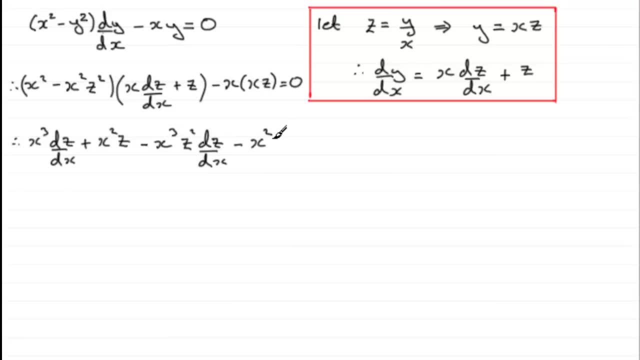 So that's going to be minus X squared Z, cubed. And then we've got this last term here, minus X squared Z, And that equals zero. So what I notice is that these two terms here minus X, squared Z, squared times X squared Z, squared. 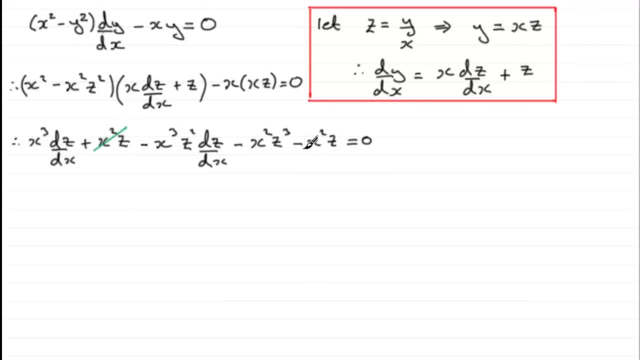 these two terms, x squared z and minus x squared z. well, they're going to give a zero there, and what I can do now is group together these two terms containing dz, dx. I can pull out x cubed as a common factor as well, so therefore, what we've got is x cubed multiplied by one. okay, I'm going. 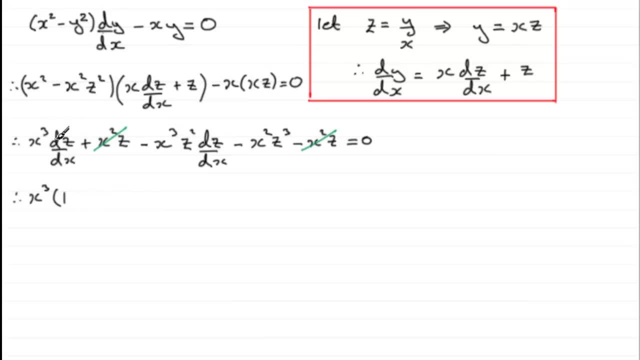 to put dz dx at the rear of this bracket here. so I've got x cubed times one and I've got minus and then just the z squared and then write the dz by dx at the rear of the bracket. okay, always a good position for writing dz dx at the rear brackets rather than at the front. 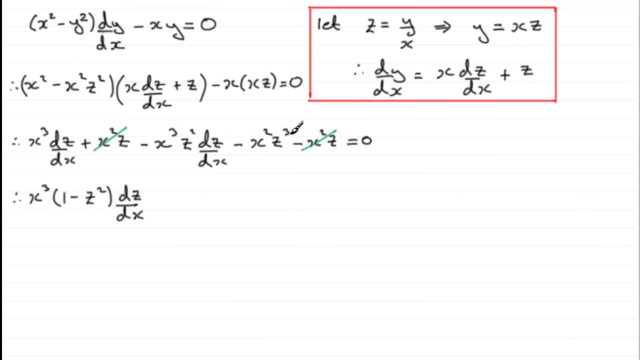 and now I'm just going to add x squared z cubed to both sides, so I get equals x squared z cubed and I can see that this differential equation. now I can separate the variables. I can get all the z's on one side and all the x's on the other side if I divide both sides by z. 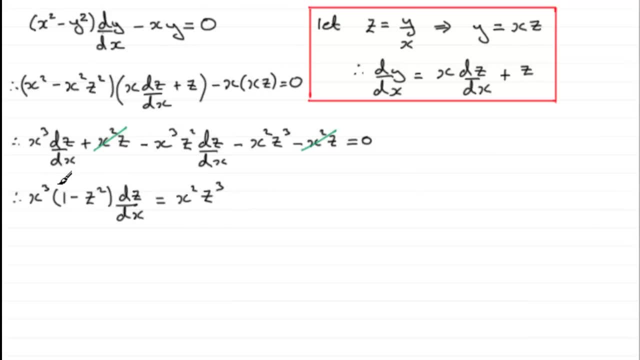 cubed and divide by x cubed and rearrange this with the dx over here, I end up with one minus z squared over z cubed, dz equals and then x squared divided by x cubed is going to be one over x and then that'll be dx and I can integrate both sides so okay. so that's separating the. 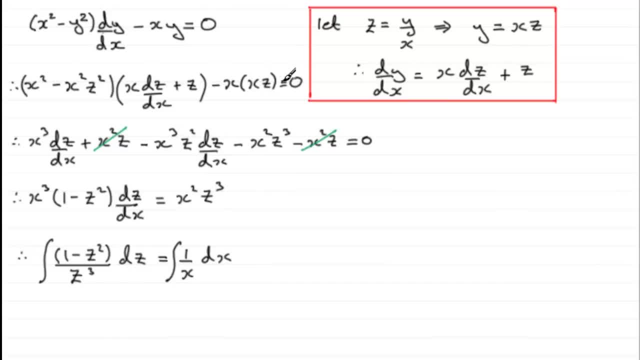 variables there. so with this substitution, then that's good. it just allows me to do that, allows us to get into this form now, and you might even like to pause the video at this stage and just carry on and complete this example. just give you a few moments if you'd like to do that. 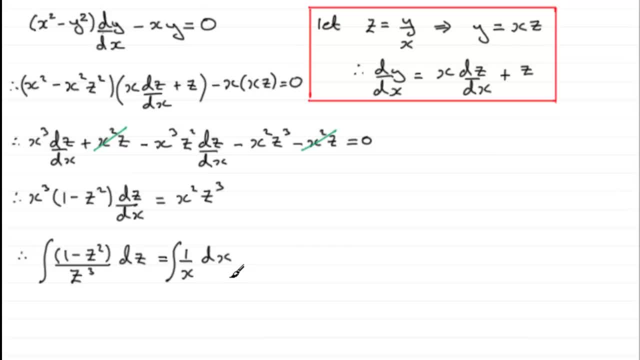 okay, welcome back. if you did carry on with this. well, here's the next part. anyway, what we can do here is think of this as being the integral, then, of one over z cubed, which is z to the power minus three, and then z squared over z cubed. that's going to be. 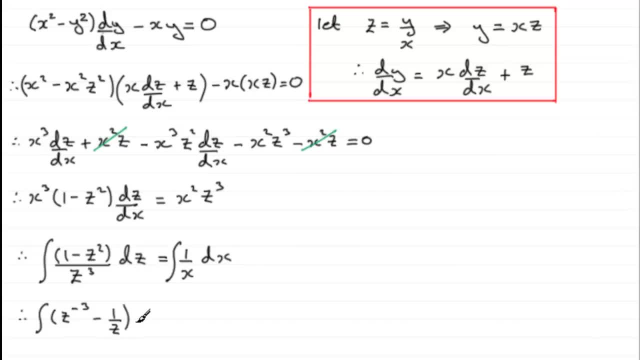 minus 1 over z, and we're integrating this with respect to z and we've got on the other side the integral of 1 over x with respect to x. now, if I just border this off, okay, we come around here looks a bit ugly, unfortunately, but it'd be just good to keep this on the same screen. well, 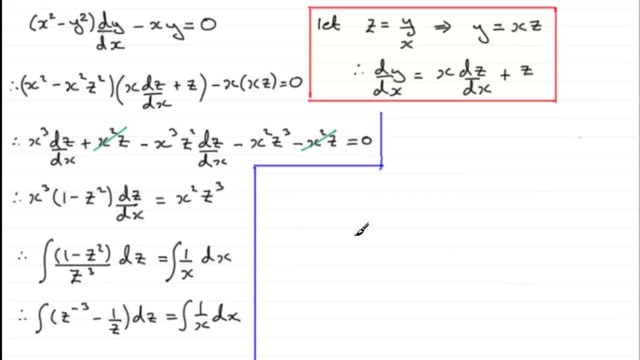 the integral of z to the power minus 3. that's going to be z to the minus 2 all divided by minus 2, and then we've got the integral of minus 1 over z with respect to z, so that's going to be minus the. 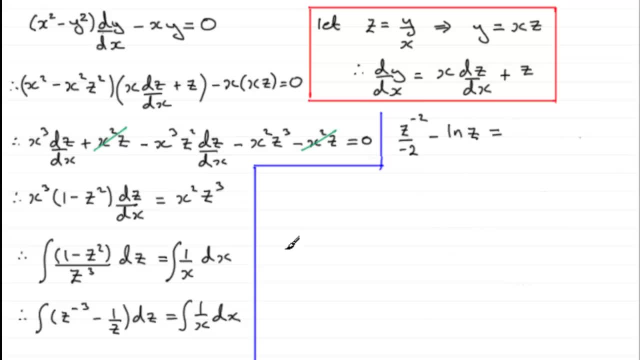 natural log of z, and then equals and the integral of 1 over x with respect to x. well, that's going to be the natural log of x. and then don't forget the constant of integration plus c. now we need to get our answer in terms of x's and y's, so we need to substitute for z as y over x. so if we make 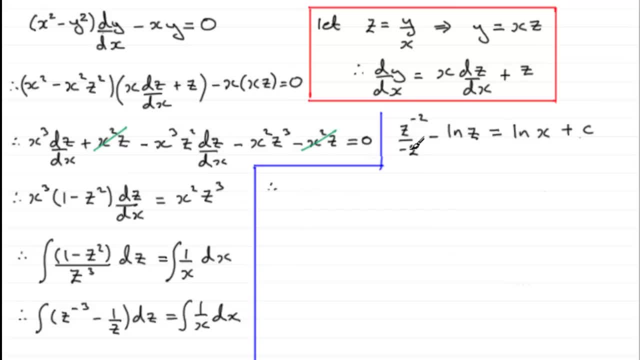 that substitution we therefore have. well, this is going to be minus 1 over 2 z squared, and so when we make that substitution, we'll end up with inverting this fraction here, so it'll turn out to be minus x squared over z squared. so that's going to be minus 1 over 2 z squared. so that's going to 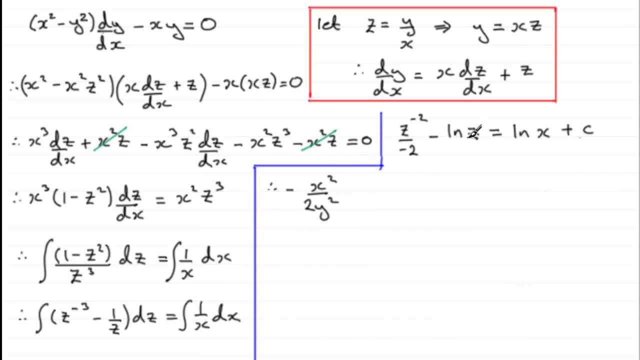 be minus 1 over 2 y squared, and then we've got minus the natural log of z, which is y over x, and then equals the natural log of x plus the constant of integration plus c. so what I could do now is just remove the 2y squared by multiplying throughout by 2y squared, and also you. 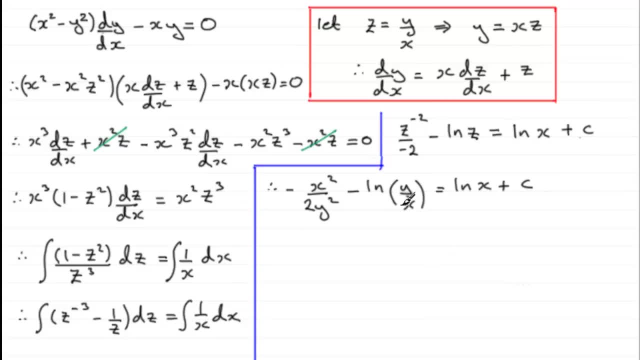 just remove the 2y squared by multiplying throughout by 2y squared and also you changing this to the natural log of y minus the natural log of x. so if we do that, we therefore have got minus x squared and then minus 2y squared. 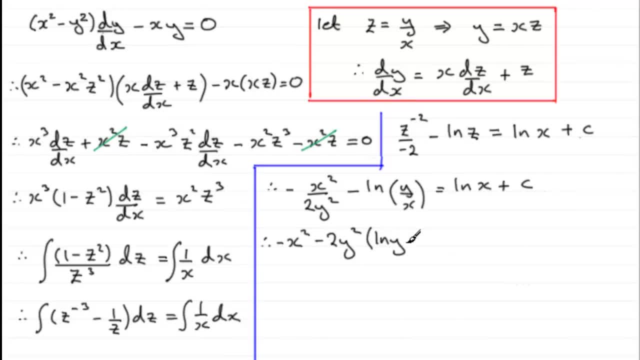 multiplied by the natural log of y minus the natural log of x, and that will equal. well, remember, we've got to multiply this term by 2y squared, so we've got 2y squared natural log of x. and we've also got that constant c to multiply with the 2y squared, so we've got 2y squared times that constant c. 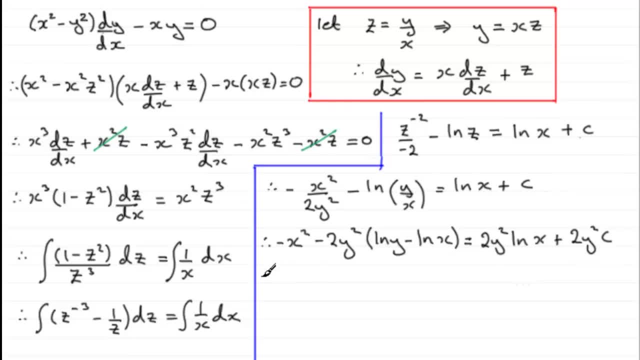 let's expand the bracket here, so we therefore have minus x squared minus 2y squared natural log of y plus 2y squared natural log of x equals 2y squared natural log of x plus 2y squared times c, and I can see that 2y squared natural log of x occurs here and here, so that 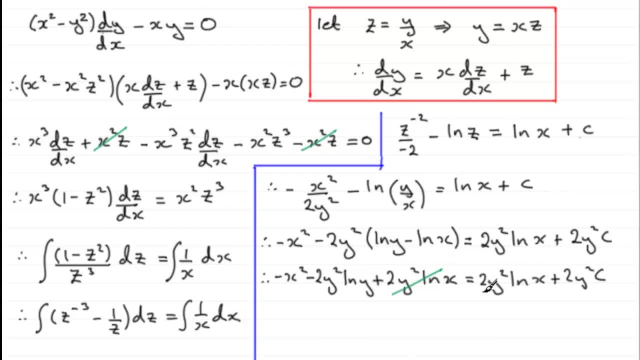 when I subtract that from both sides, that's going to disappear. so if I add x squared and 2y squared natural log of y to both sides, then I can pull out 2y squared as a common factor between this term. so be natural log of y and we've 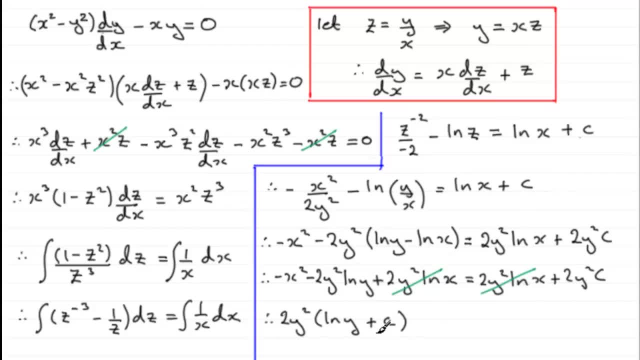 got this term down here- plus c, okay, and then if I add the x squared as well to both sides, we've got plus x squared and it will equal 0. so there you go. a general solution, then, to our differential equation. just by making this substitution, it helped us change the form of this into one that involved: